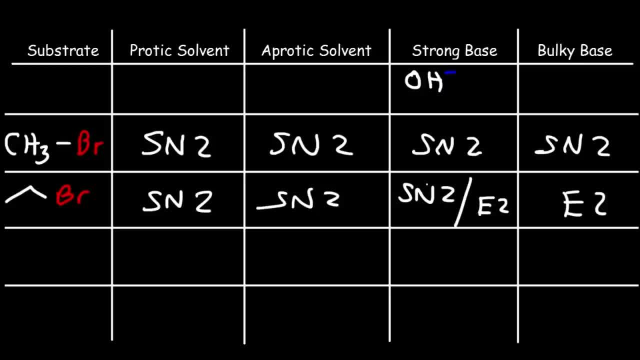 But if the substrate is not hindered- sterically hindered- then it's going to be SN2.. Let's say, if you use a strong base like hydroxide or even methoxide- Now, ethoxide would also fit this category- 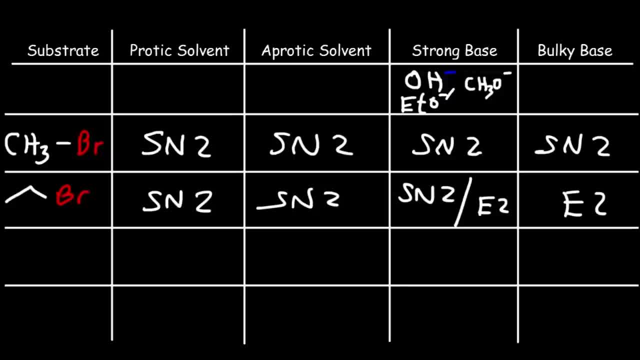 So we see ET, that's ethyl CH3CH2.. One good example of a bulky base would be tert-butoxide, And so if you react it with a primary alkyl halide, you're going to get an E2 reaction. 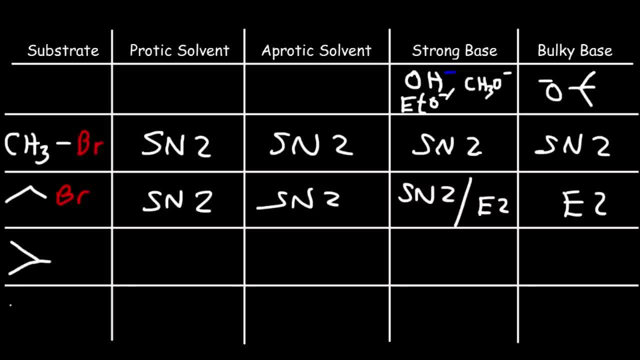 Now if we have a secondary alkyl halide, that's when things can get interesting. So if you use an aprotic solvent, such as acetone or DMF or DMSO, with a very good nucleophile like iodide cyanide or a sulfur with a negative charge, this is going to favor the SN2 reaction. 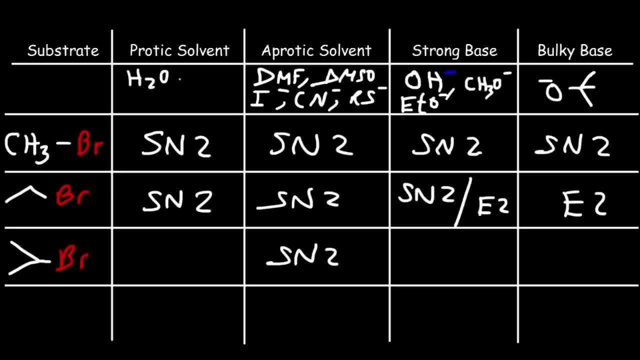 Now, if you use a protic solvent Like water or methanol or even ethanol, where you have hydrogen bonds, Typically this will favor the SN1 and the E1 mechanism, But this can vary too. Sometimes it could favor an SN2 reaction. 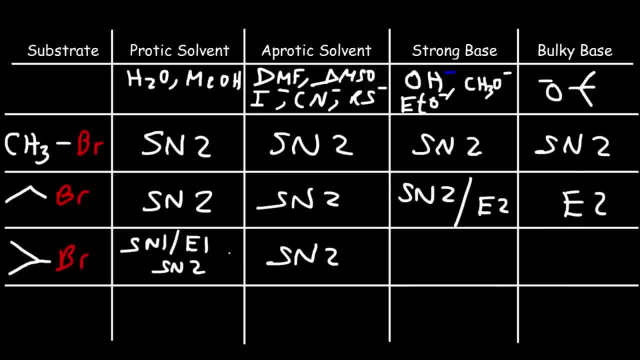 So you got to pay special attention to this category. But the protic solvent favors the SN1 and the E1 mechanism over the SN2 mechanism. Now what mechanism? It will occur if we use a secondary alkyl halide with a strong base. 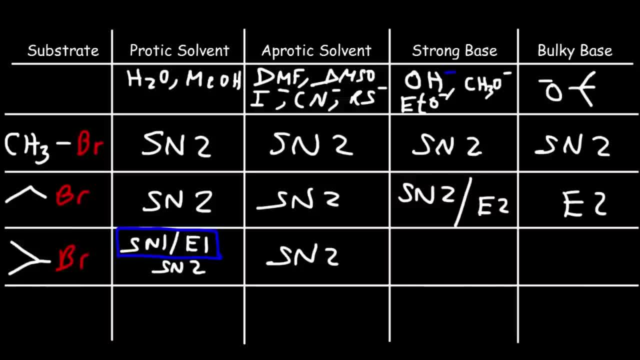 In this case you can get both the SN2 mechanism and the E2 mechanism. However, the E2 mechanism will usually be the major product. So if you have a bulky or sterically hindered secondary alkyl halide, it's going to favor the E2 reaction over the SN2 reaction. 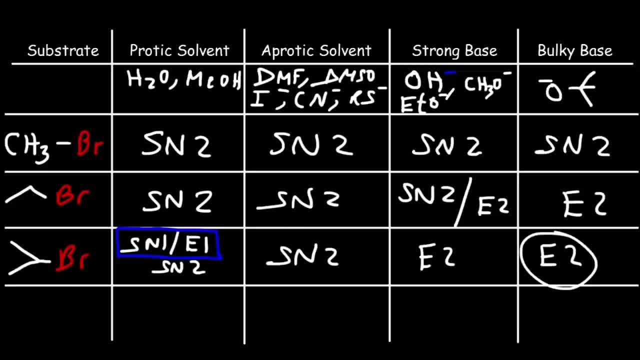 And using a bulky base will also favor E2 over SN2.. However, if you use a secondary alkyl halide with a strong base, you can get both the SN2 mechanism and the E2 mechanism. However, if you have, let's say, hydroxide and a secondary alkyl halide, that's not sterically hindered. 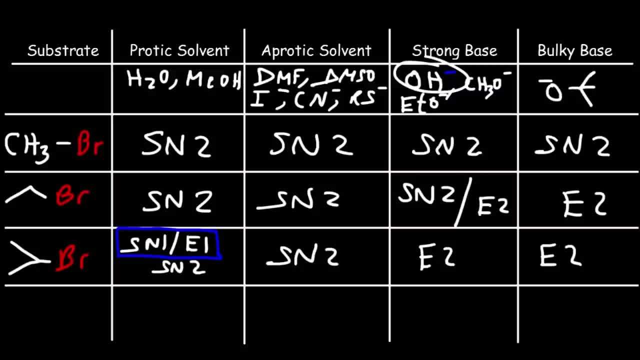 then you can get a good mixture of the SN2 reaction and the E2 reaction, But typically the E2 will slightly be. You'll get the E2 in a better yield over the SN2.. But you'll still get a good mix of both of them. 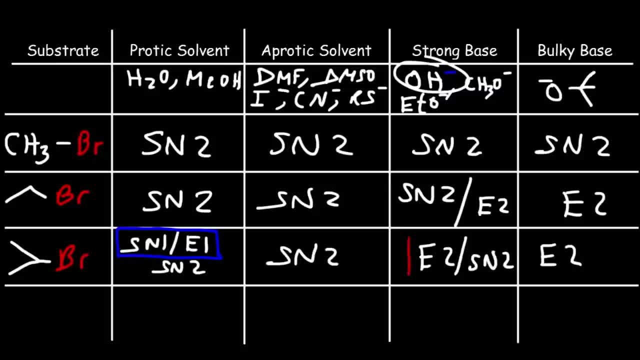 So I'm going to put the E2 on top here because this is going to be the major product, But know that the SN2 reaction still exists in this category. It's simply the minor product. Now, if we have a tertiary alkyl halide, we're not going to get the SN2 reaction because it's too sterically hindered. 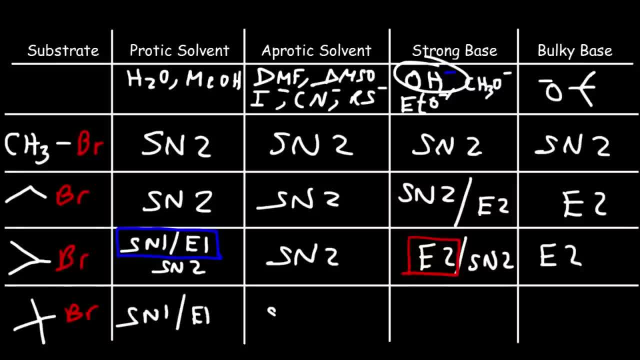 And so we're going to get the SN1 and the E1 reaction, regardless of the solvent that we choose to use. Protic solvents favor the SN1 reaction, A-protic solvents favor the SN2 reaction, And heat favors E1 over SN1,, by the way. 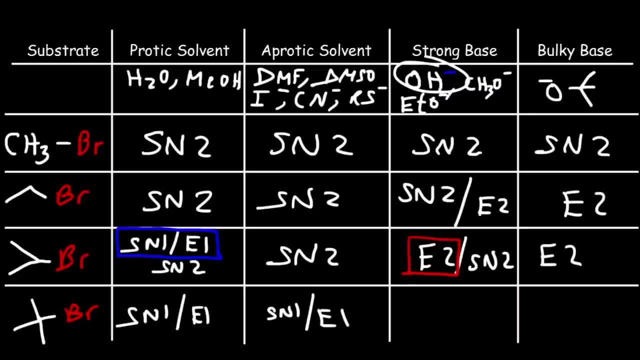 So if you wish to increase the E1 yield over the SN1 yield, you need to raise the temperature. Using a strong base with a tertiary alkyl halide will favor the E2 reaction. You're not going to get the SN2 reaction. 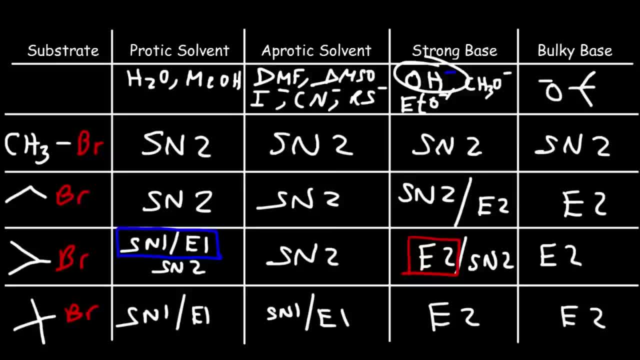 So this table is not perfect- There are exceptions, But this is simply a general guideline to help you predict Which mechanism will be the major pathway in a substitution or elimination reaction. So let's go ahead and work on some examples. So let's start with this one. 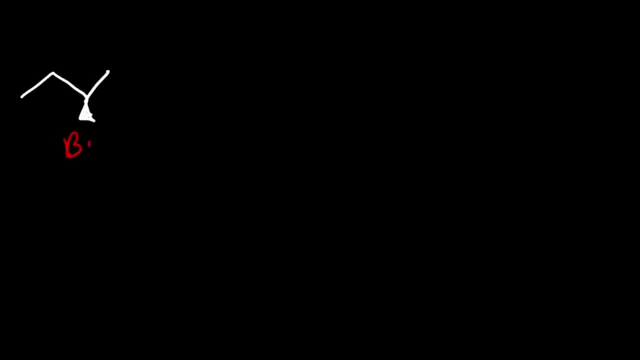 2-bromobutane And let's react it with Sodium, cyanide And acetone. So which mechanism Will this reaction proceed with? Is it going to be SN1, SN2,, E1, or E2?? 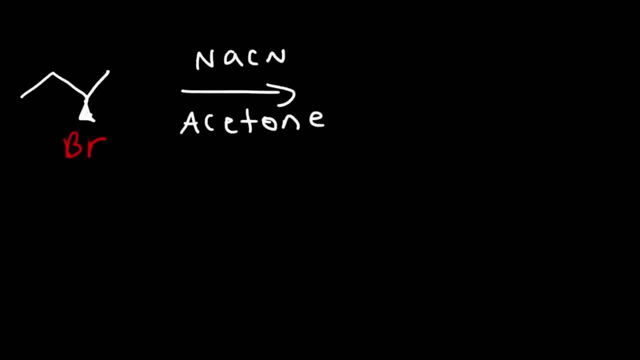 And then, once we know the mechanism, let's predict the major product and show the mechanism to get to that product. So we have a secondary alkyl halide, The carbon that bears the bromine atom. That carbon is attached to 2 other carbon atoms. 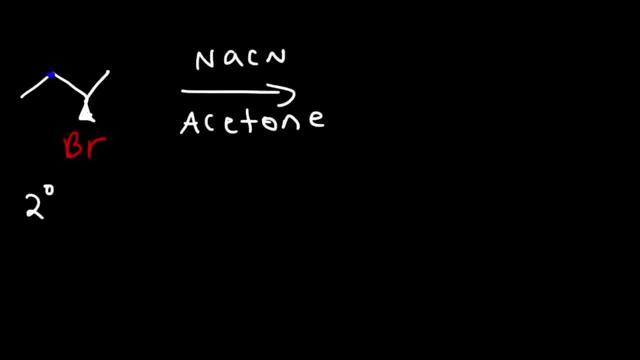 So we have a secondary alkyl halide. Now the cyanide Ion Is the secondary alkyl halide And the carbon is attached to 2 other carbon atoms. So we have a secondary alkyl halide, Now the cyanide. 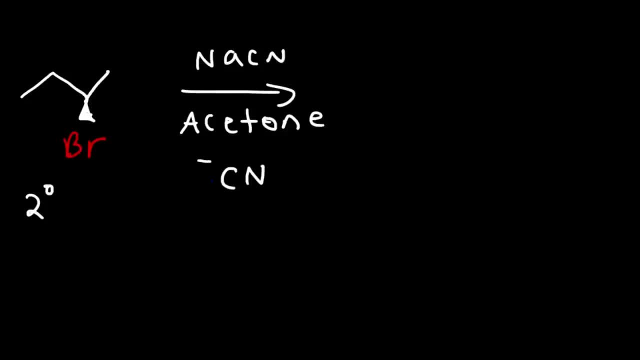 Ion, the nucleophile, in this reaction, And so the nucleophile is going to attack the carbon from the back- also known as the backside attack- and it's going to expel the leaving group. Because it attacks from the back, we're going to get the inverted product, So the SN2 reaction. 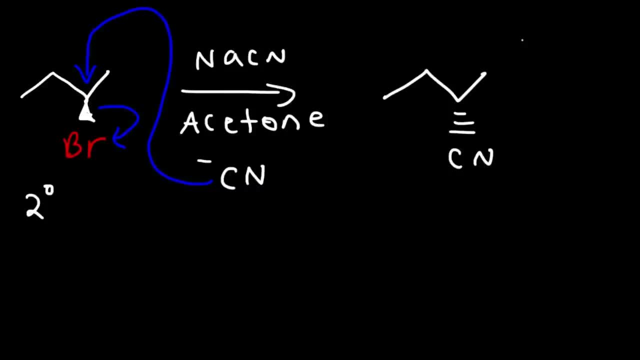 proceeds with inversion of configuration. And so here on the left side, we have the R-isomer. This is R-2-bromobutane, and now we have the S-isomer. Now let's move on to our next example. 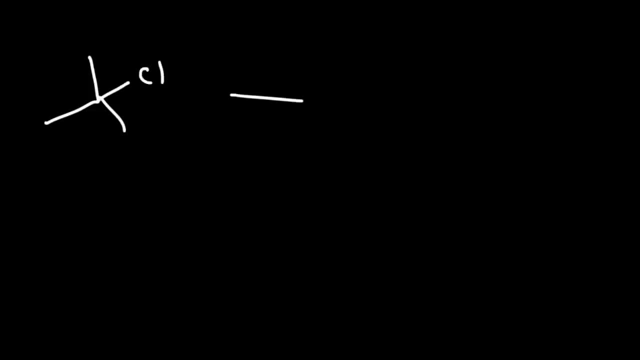 Let's say we have tert-butyl chloride and let's react it with water, Go ahead and predict the major product for this reaction. So first we need to identify the mechanism. This carbon is tertiary, so we have a tertiary alcohol, So we have a tertiary alcohol. So we have a tertiary alcohol, So we have a tertiary. 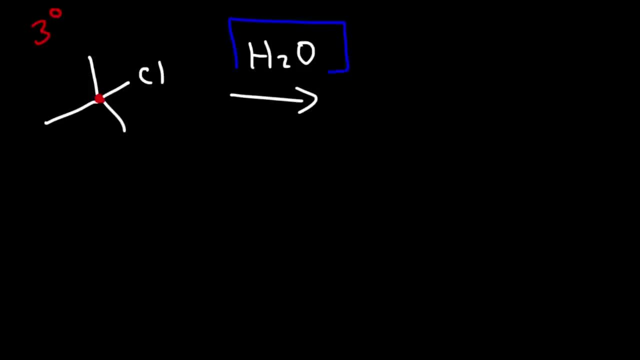 tertiary alcohol. So we have a tertiary alcohol. So we have a tertiary alcohol, So we have a tertiary chloride And we have a protic solvent, H2O. So the dominant mechanism will be the SN1 and the E1 mechanism. So let's draw the products for the SN1 mechanism and for the E1 mechanism. SN1 stands for 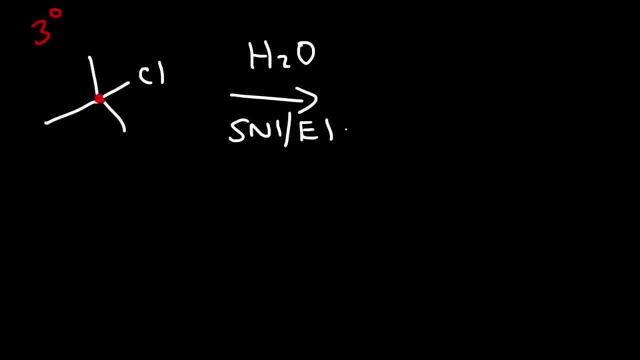 the first-order nucleophilic substitution reaction, And so we're going to replace the chlorine atom with an OH group. In an E1 reaction or elimination reaction, we're going to remove a hydrogen and the leaving group, forming a double bond or an alkene. Now the first step for the SN1 reaction. 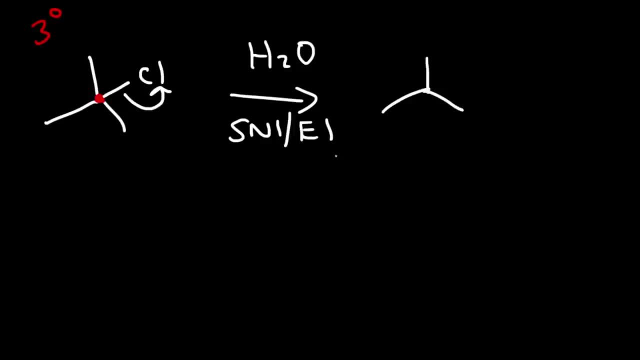 is that the leaving group leaves, And so we're going to get a tertiary carbocation, And then the water molecule is going to add to this tertiary carbocation, And so we're going to get this oxonium species, And then we need to use another water molecule to take off a hydrogen. 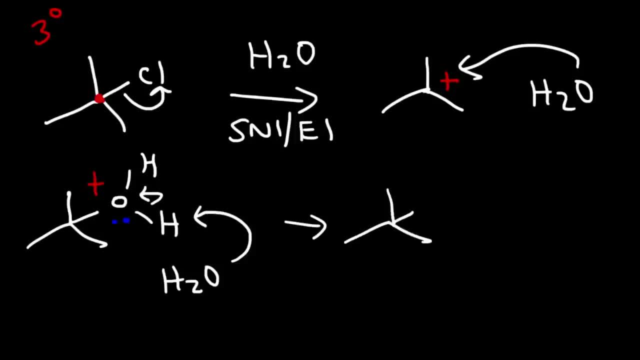 So the end result is an alcohol, And so this is the SN1 product for this reaction. Now let's draw the E1 product for that reaction. So the first step in the SN1 reaction and the E1 reaction is the same, and that is ionization, The leaving group. 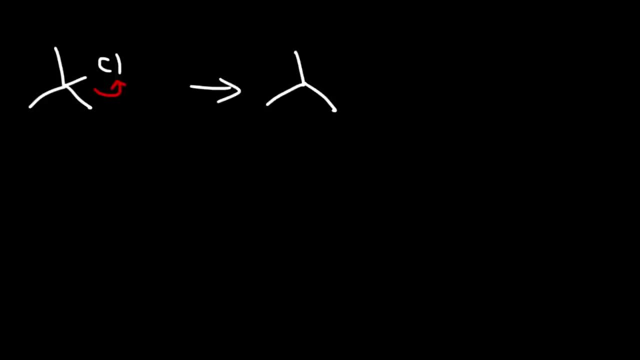 is going to leave and we're going to get the same tertiary carbocation. Now for the E1 mechanism. this is where the path changes compared to the SN1 mechanism. For the E1 reaction, the water is not going to act as a nucleophile attacking the carbocation. 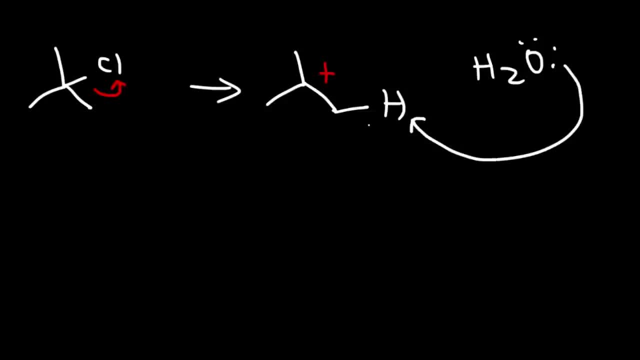 Instead, it's going to act as a base, going for the hydrogen, and then the carbon hydrogen bond will break. Those two electrons will be used to form the pi bond, given us an alkene. So that's the E1 mechanism. Now let's try this example. 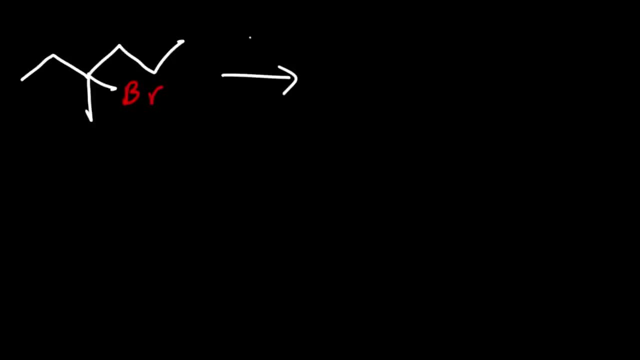 Let's react this alkyl halide with methanol. Go ahead and predict the products of this reaction. So on the left we have a tertiary alkyl halide and we have a protic solvent. When the solvent acts as a nucleophile, it's called a solvolysis reaction. 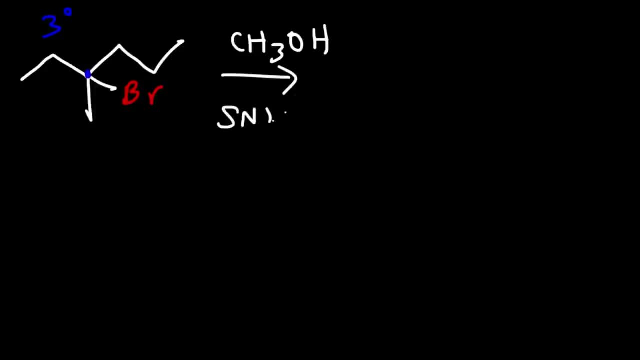 And when you see that it's typically an SN1- E1 reaction. So let's focus on the SN1 product. The SN1 reaction is a substitution reaction, So we're going to substitute the leaving group with this group, and we're going to get rid of the hydrogen, So we're going to get an ether. 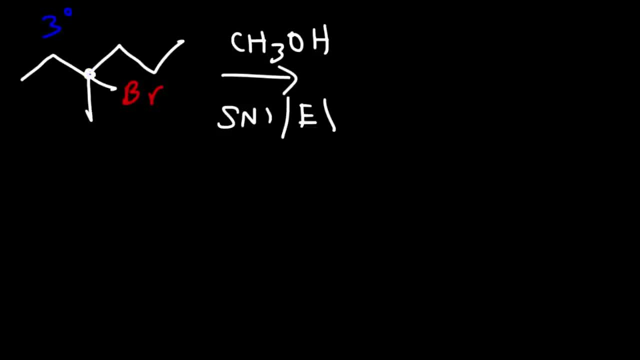 However, notice that this carbon is chiral, and so we're going to get a mixture of stereoisomers. So the OCH3 group. it can be in the front, it could be on the wedge or it can be on a dash. So these are the SN1 products for this reaction. 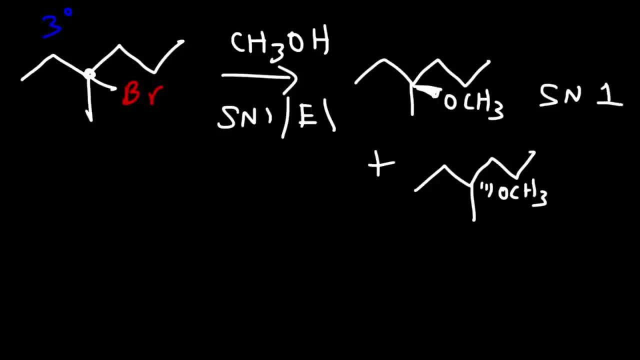 Now let's talk about why we can get a sterio isomer. Now let's talk about why we can get a sterio isomer, Why we get this racemic mixture, Why we get this racemic mixture. Well, we know, the first step is ionization. 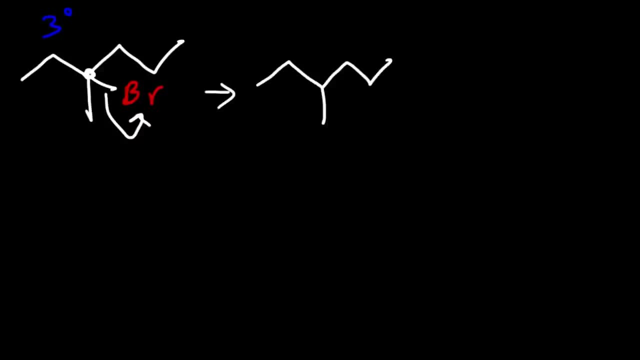 So this will produce a tertiary carbocadine. Now the methanol molecule is going to act as a nucleophile And notice that it can approach the carbocadine from either side. It can go from the back, leading to the inverted product. 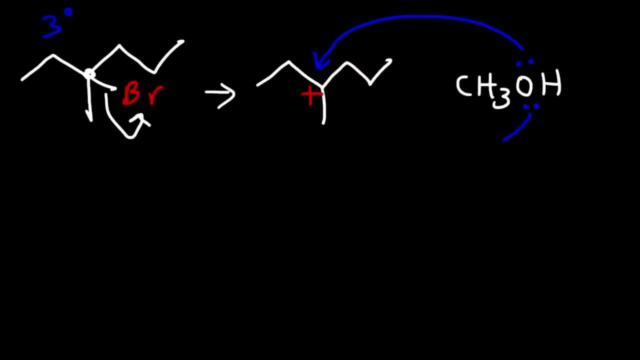 product, or it can go to the front, which is retention. so let's say, the bromine atom is in the front or on the wedge. so if it attacks from the back, we're going to get this, the inverted product. if it attacks from the front, we're going to get retention. now, of course, there's 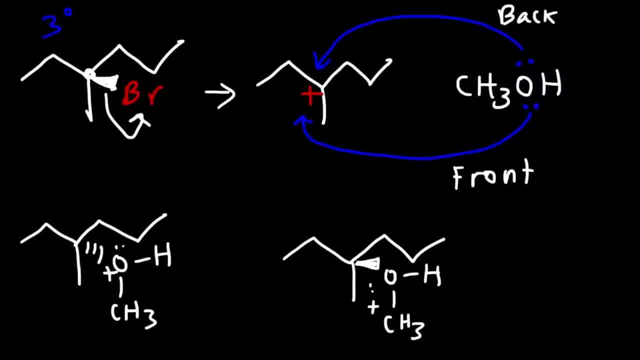 one more step. we need to take off the hydrogen. but will we get an equal amount of the inverted product and the retention product, or will one stereoisomer have a greater yield over the other? now the bromide ion is still in the vicinity of the carbocation, and so when the methanol 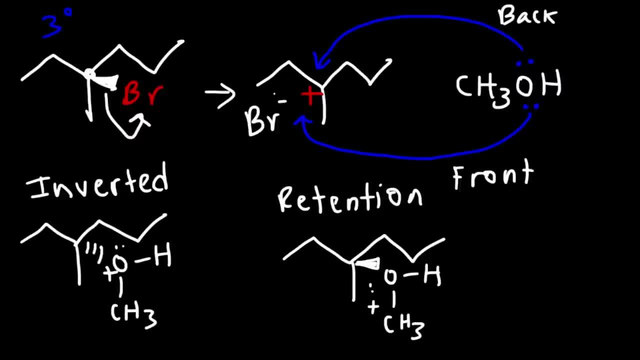 molecule approaches from the front, it's going to be repelled by the negative charge of the bromide ion. keep in mind that the oxygen atom has a partial negative charge and so it's repelled by the bromide ion. therefore, we're going to get a lower yield of the retention product. 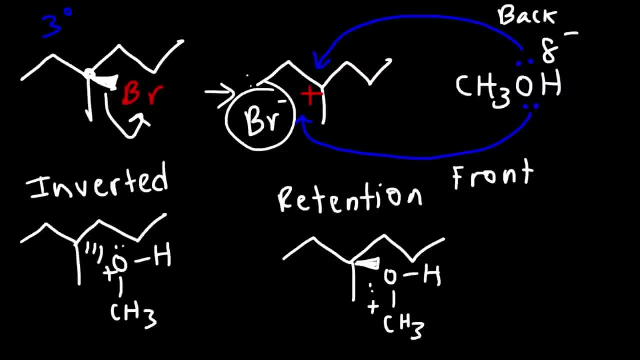 than the inverted product, so the backside attack is still more favorable. so it could be 60% of the inverted product and 40% of the retention product, or it could be a 70-30 ratio. either case you get slightly more of the inverted. 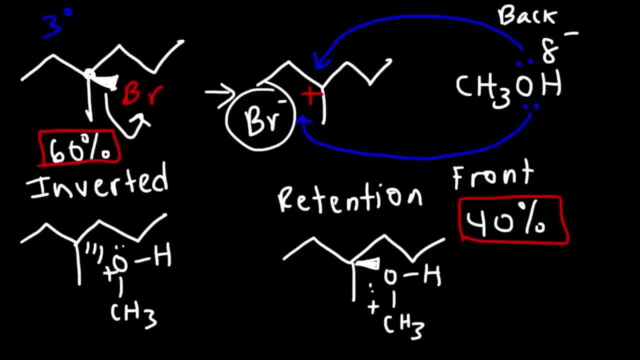 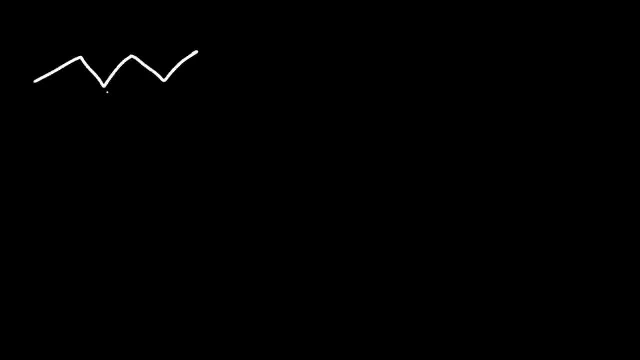 isomer as opposed to the retention stereoisomer. now for the last step of the mechanism. all we need to do is use another methanol molecule to remove the hydrogen, and so this will give us our ether product. so one is going to be on the wedge and the other will be on a dash. now let's focus on the e1 reaction feel. 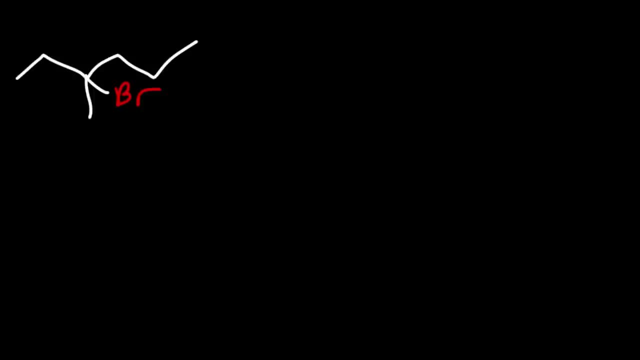 free to pause the video and write a mechanism for the e1 reaction. so the first step is ionization, and this will give us our tertiary carbop Hui guy. now, in the next step for the e1 reaction, methanol is going to act as a base instead of a Nucleus, so it's going to 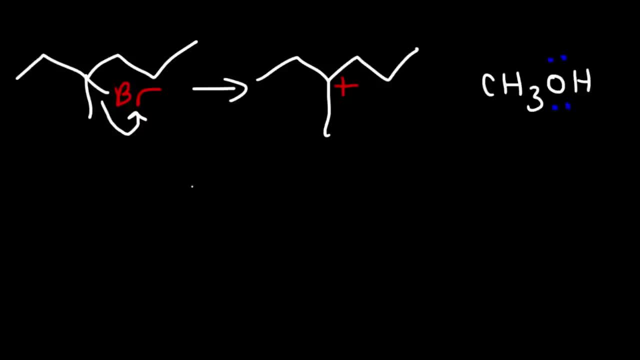 abstract: one hydrogen away from the Carmelbright noodles within your, so the hydrogen has to be one carbon away from the car boot. FL standee can take the white hydrogen hydrogen as an example here, either to the blue hydrogen or to replace it to white hydrogen质. 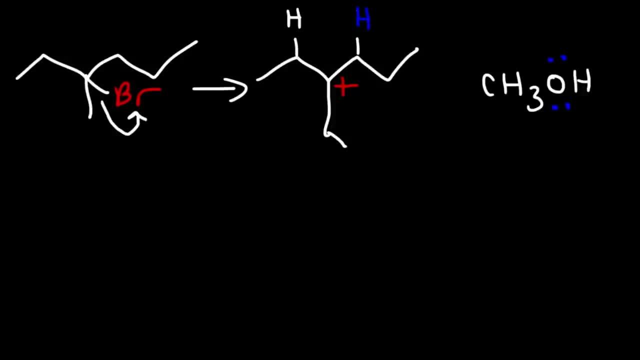 blue hydrogen质 Or it can take the green hydrogen. So if it takes the green hydrogen, we can get this product. Now, if it goes for the blue hydrogen, we can get this product, And if it goes for the white hydrogen, we can get this product. 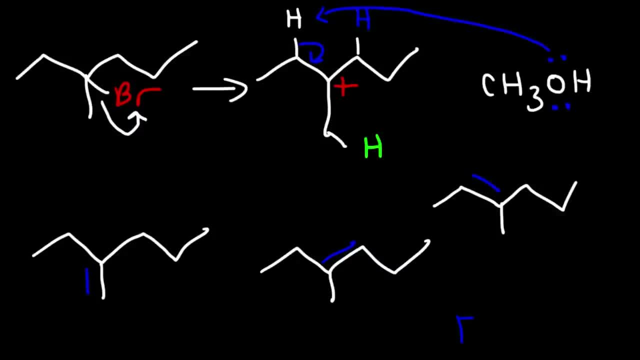 And so we get a mixture of E1 products for this reaction. However, not all of these alkenes are equally stable, So this particular alkene is a mixture of E1 products. This alkene is a disubstituted alkene. 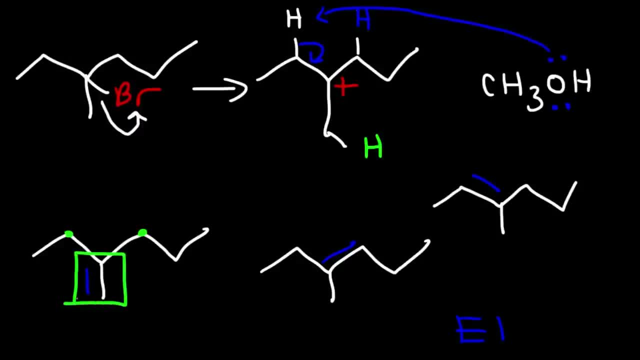 There's two carbon atoms that are attached to the two double-bonded carbon atoms. This alkene is trisubstituted, and the same is true for this one. It has three R groups, And so this is the least stable alkene. 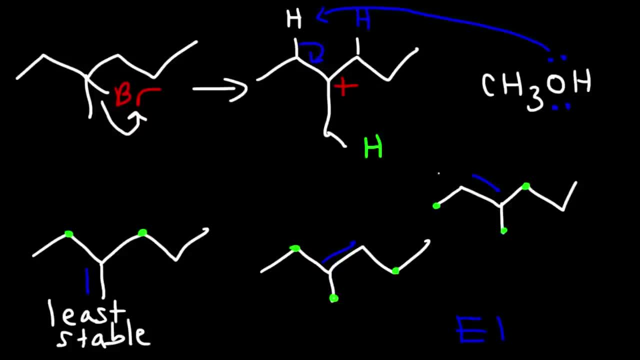 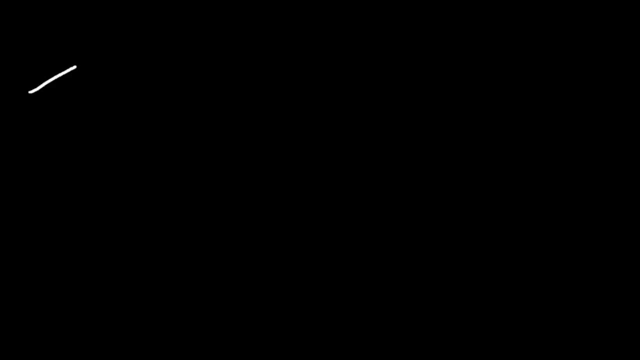 So therefore, the major product for the E1 reaction will be these two alkenes. They will both form in good yield. This will be the minor E1 product. Now, let's say, if we have 2-bromo-3-methylbutane. 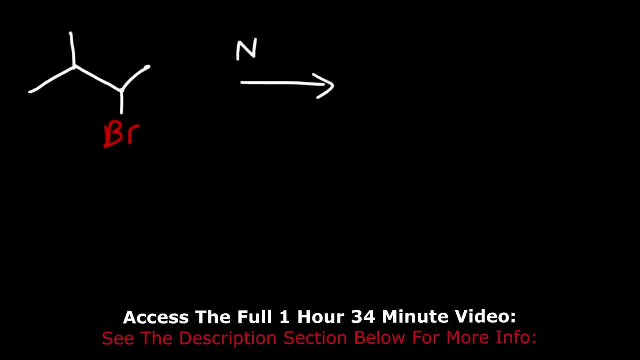 And let's react it with sodium methoxide and methanol. What is the major product in this reaction? Go ahead and try it. So we have a secondary alkyl halide And methoxide. Methoxide is a strong base. It's not a sterically hindered base, but it is a strong base. 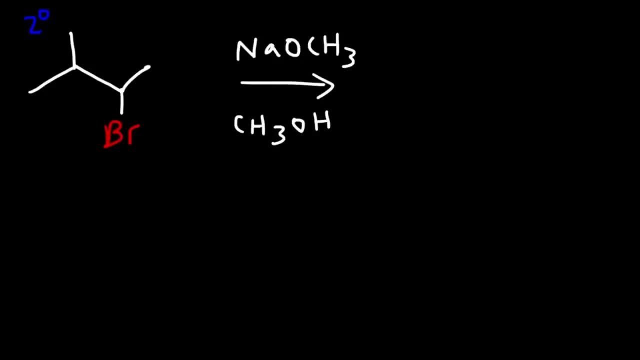 And so whenever you have a secondary alkyl halide with a strong base, the major product is typically the E2 product And the SN2 reaction will give you the minor product, But we're going to draw both. So let's start with the SN2 reaction. 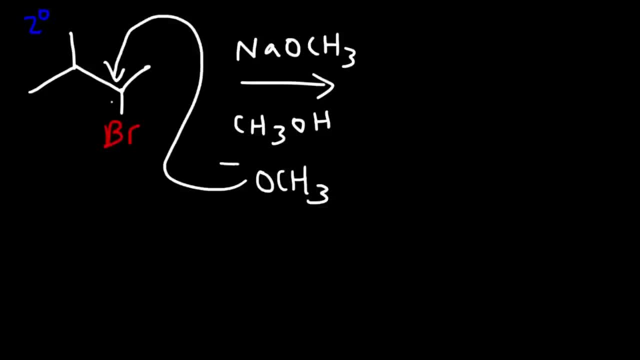 So the methoxide will attack this carbon, Kicking out the bromine atom. Now we don't have to worry about the stereochemistry, because it wasn't specified at this carbon, Even though we could get a mixture of stereoisomers, Because this compound could be R or S. 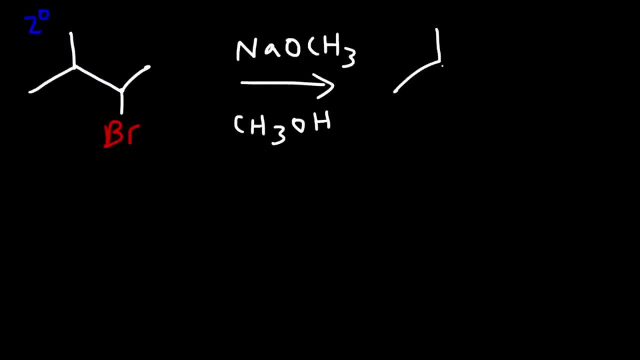 We don't know, But we're not going to worry about stereochemistry. The SN2 reaction will give you the inverted product. So let's say, if this was in the front, Then the OCH3 group would have to be In the back. 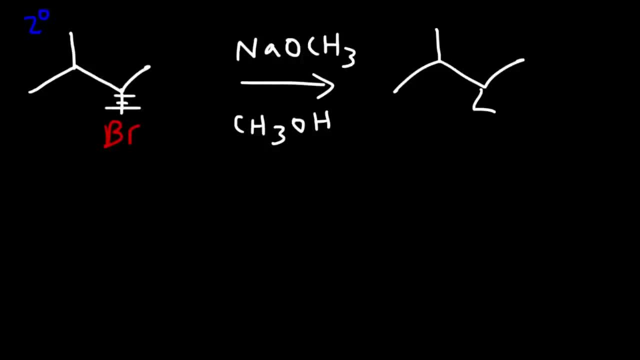 Or if this was in the back, Then the OCH3 group will have to be in the front. So since the stereochemistry wasn't specified, We're not going to specify it here either. So this is going to be the SN2 product. 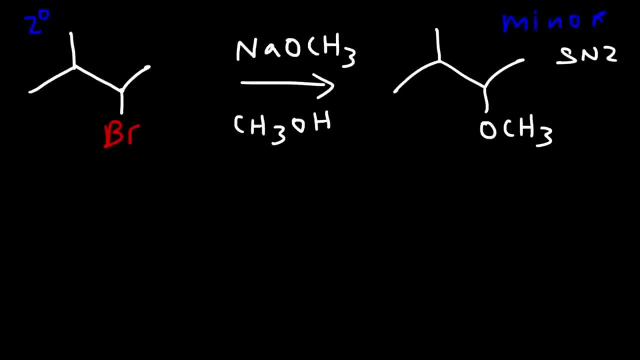 And this is going to be the minor product in this reaction. It can happen, but it's not going to be in good yield. Now for the E2 reaction. No rearrangements can occur. The base can take off a hydrogen, one carbon, away from the carbon that bears the bromide atom. 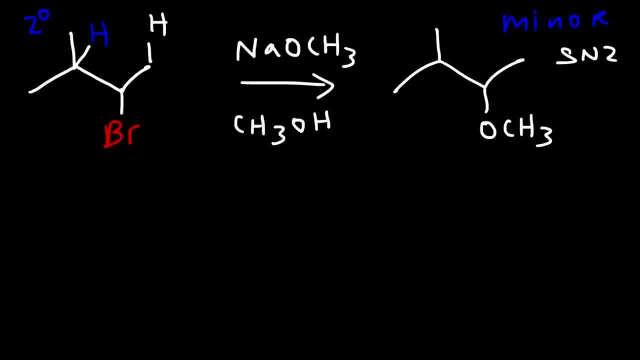 So it can take the white hydrogen or the blue hydrogen. Methoxide will preferentially take the blue hydrogen over the white hydrogen, And so we're going to get this particular E2 reaction. So this is going to be the major E2 product. 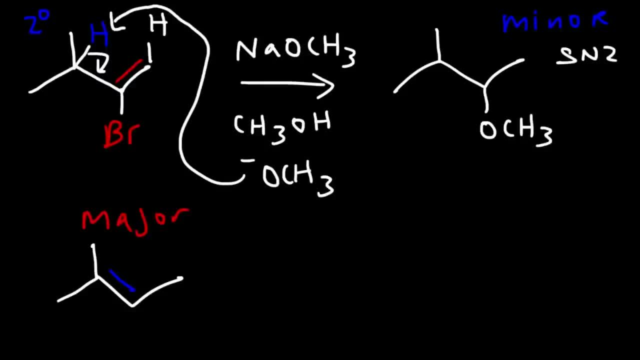 Now it could take the white hydrogen, Put in a double bond here, And this will be the minor E2 product. Now you need to know that internal alkenes are generally more stable than terminal alkenes, So this alkene here is more stable than the one on the right. 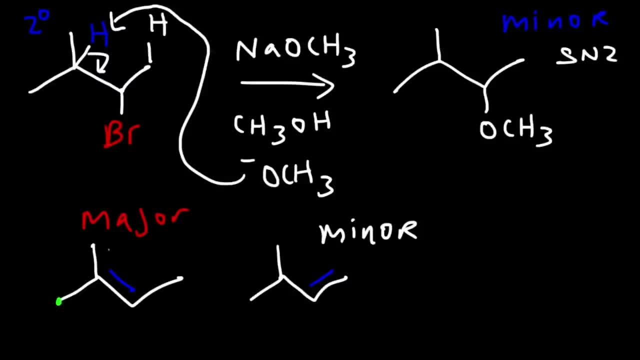 And the reason being is it's more substituted. Here We have a Tri-substituted alkene. On the right, There's only one carbon attached to these two double bonded carbon atoms, And so this is a mono-substituted alkene. 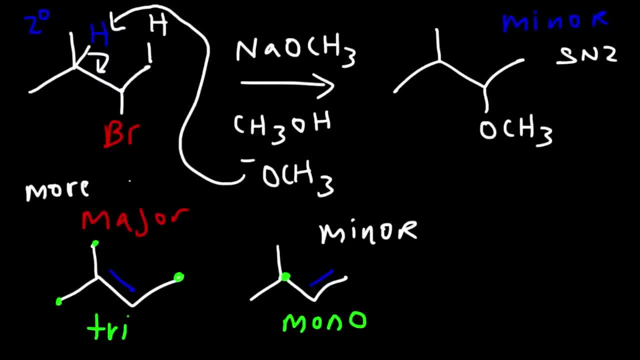 Tri-substituted alkenes are more stable than mono-substituted alkenes, And so that's why this is the major product. It's simply the more stable alkene. The most stable alkene is known as the Zetsev product. 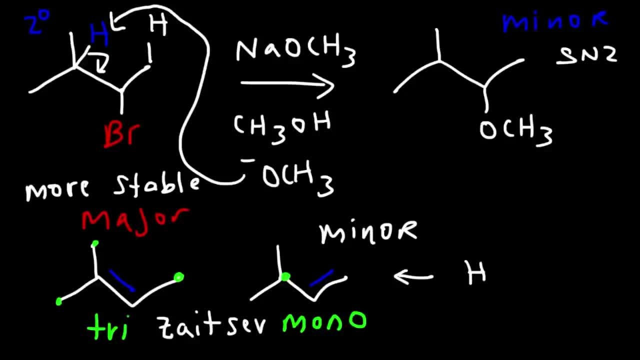 Whereas the less stable Alkene Is known as the Hoffman product, And so this is the answer For this problem. So the major mechanism for this reaction is the E2 mechanism And this is the major product overall. Keep in mind, the SN2 reaction can occur. 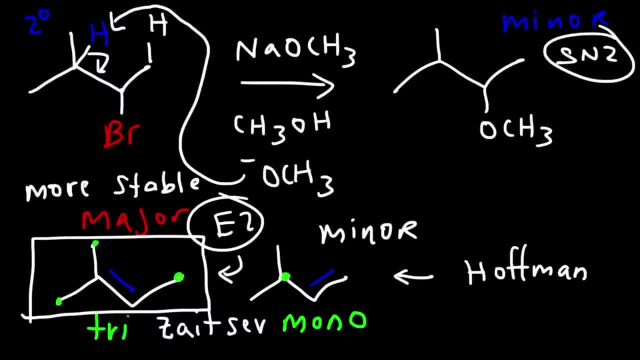 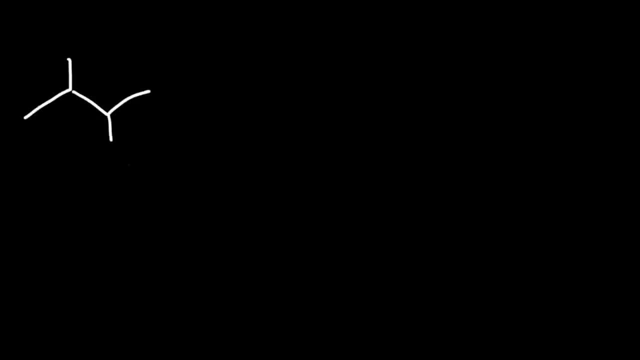 For this particular problem, But it will lead to a minor product. Now, let's say, if we have the same Alkohol halide, The same substrate, But this time We're going to use A sterically hindered base. 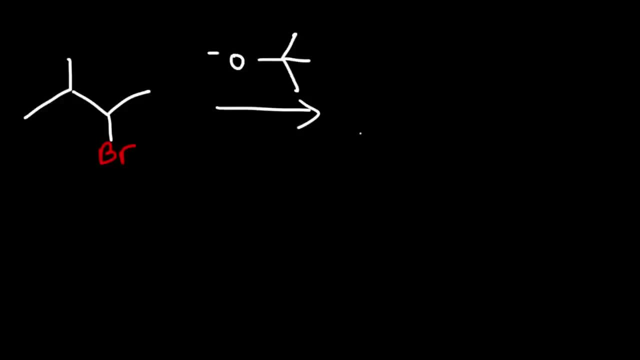 Such as Terp butoxide In terbutanol. What's going to happen? So we have a product, solvent, But we also have a strong base, And so, If you're using the triate that I mentioned in the beginning, 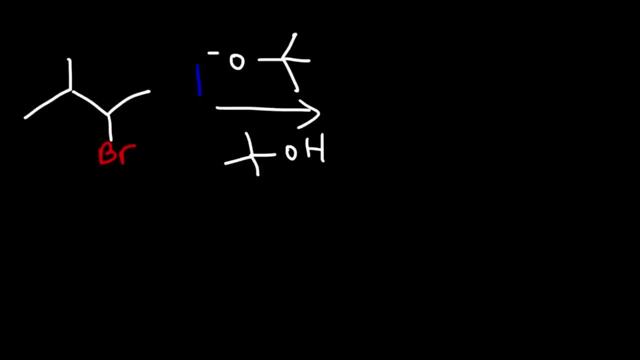 You need to use the fourth column Because the strong base Takes priority Over the product solvent, because this has a negative charge. it's far more reactive than terbunol. So we have a sterically hindered base and also a relatively sterically hindered alkyl halide. 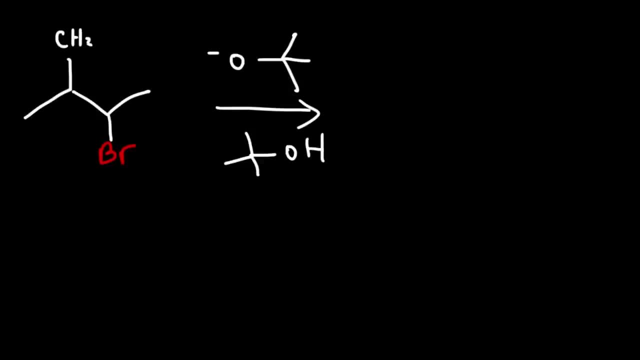 due to this methyl group on the top. So whenever you have a bulky base, an sterically hindered substrate, if both the substrate and the base are sterically hindered, this will give you the Hoffman product, and so you're going to get the less stable alkene. 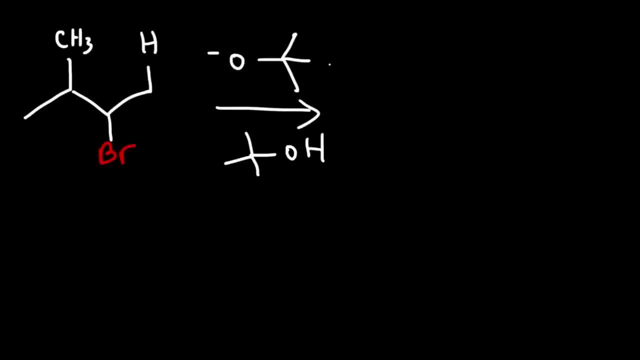 So because terbutoxide is so bulky, it wants to go for the most accessible hydrogen, And the hydrogen atoms on a primary carbon are more accessible than the hydrogen atom on a tertiary carbon. Terbutoxide doesn't want to have to struggle against these two methyl groups to get to that hydrogen. 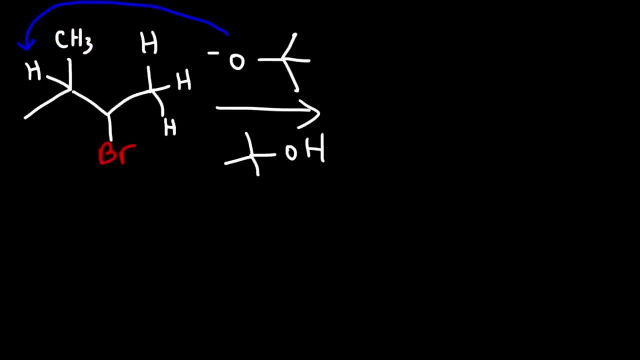 And so it's not going to. It's not going to form the Zaitsev product in good yield. It can still work, but it's going to be the minor product. Instead, it's going to go for the most accessible hydrogen atom. 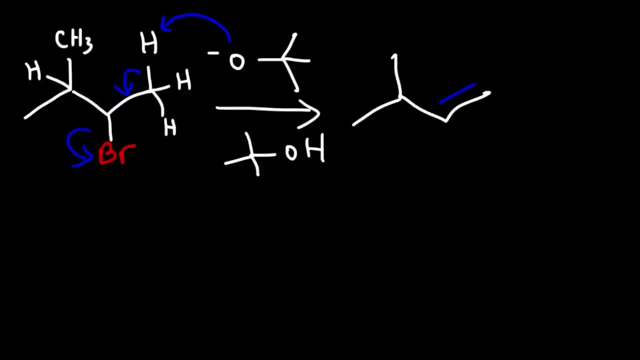 So we're going to get the Hoffman product as the major product for this reaction. Now we can still get the Zaitsev product, but it's going to be the It's going to be the minor product in this case. So the E2 reaction is the major mechanism in this example. 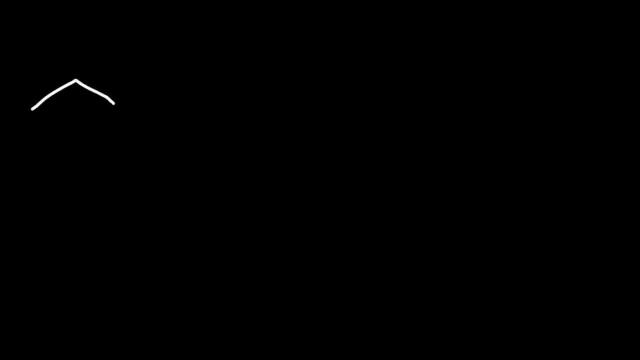 And so this is the major product. Now I want to compare these two reactions together: 2-bromopentane and 2-fluoropentane. So let's start with 2-bromopentane. I'm going to use methoxide. 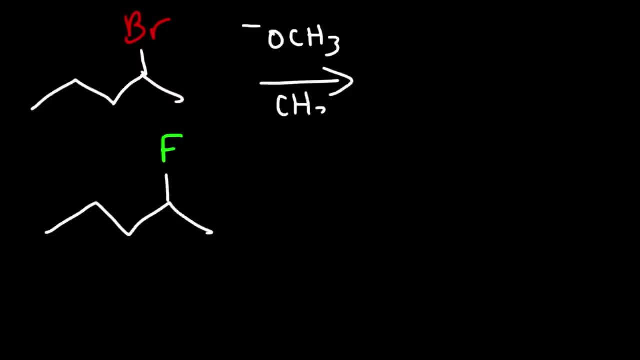 I'm going to use methoxide as the strong base dissolved in methanol, What is the major product for this reaction? So in this case, methoxide is going to go for the hydrogen, that's one carbon away from the carbon-bromine bond. 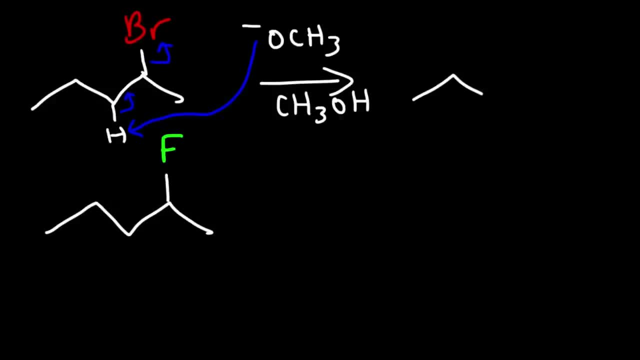 And so we're going to get the Zaitsev product as the major product. You can still get the Hoffman, but that's going to be the minor product. Now, if we use an alkyl fluoride, something different is going to happen. 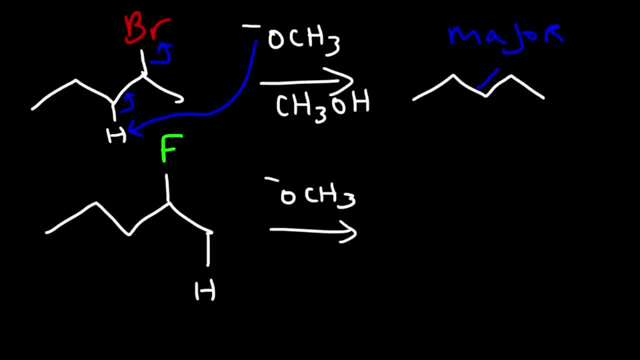 The methoxide is going to go for the primary hydrogen as opposed to the secondary hydrogen, And so we're going to get the Hoffman product as the major product. The question is why? Why do we get the Hoffman product as the major product if fluorine is the leaving group? 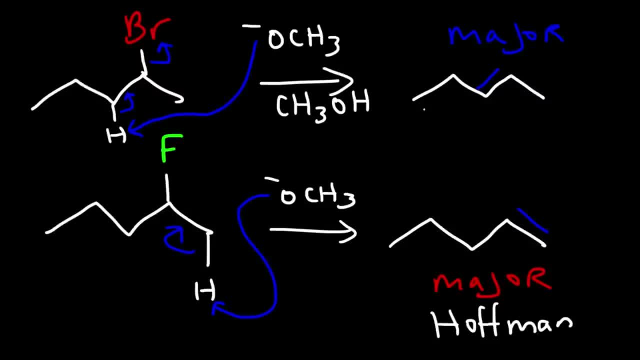 Whereas if bromine or chlorine is the major product, then we get the Zaitsev product. Why do we get the Zaitsev product as the major product? if fluorine or chlorine or iodine is the leaving group, We're going to get the Zaitsev product. 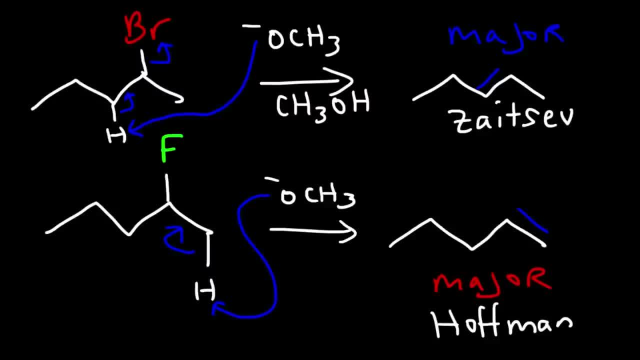 For one thing, chlorine, bromine and iodine- they're good leaving groups, And so when you have a good leaving group, it's going to favor the Zaitsev product. Fluorine, on the other hand, it's a bad leaving group. 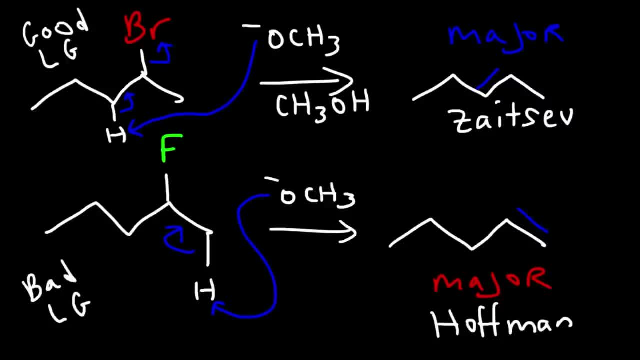 And so you're going to get the Hoffman product. Now, the reason for this is, when you have a good leaving group, the transition state resembles an alkene And so because of that, you need to find the most stable alkene. So the major product will have or will be associated with the most stable alkene. 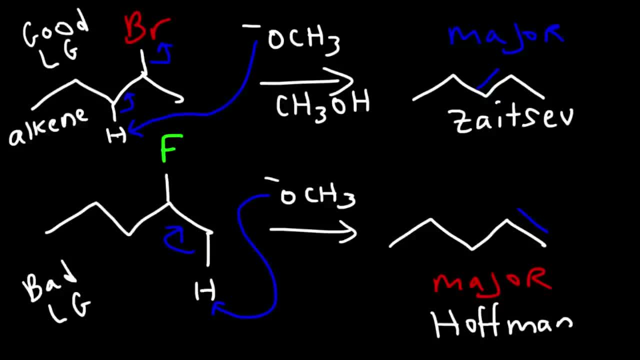 because that's going to give you the most stable transition state In the case of an alkyl fluoride. because it's a bad leaving group. when the methoxide ion approaches to attack the hydrogen, the fluorine is still sticking around. It doesn't want to leave. 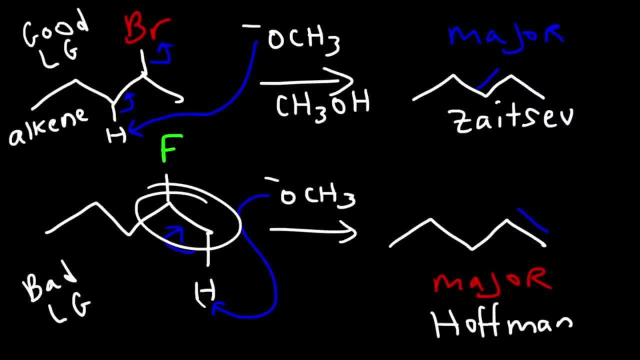 And so you have this buildup of negative charge on this molecule, And so the transition state resembles more like a carbanion instead of an alkene, And what you need to know is that primary carbanions are more stable than secondary carbanions. 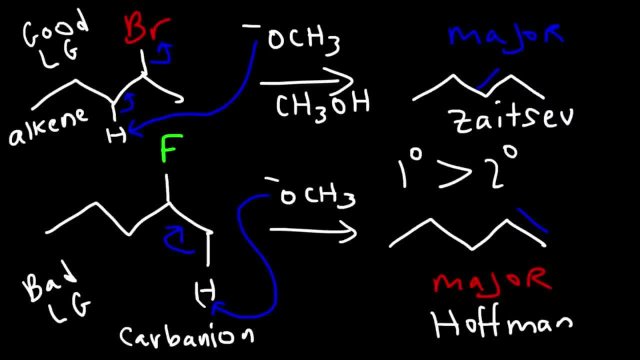 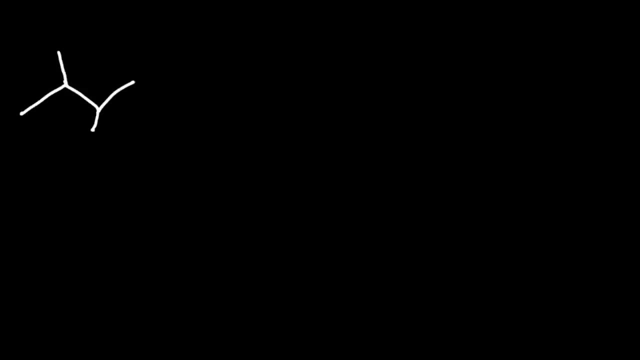 And, as a result, it's better to put the negative charge on a primary carbon as opposed to a secondary carbon, And this is why the Hoffman product is the major product. Now I want you to compare these two reaction mechanisms. Let's say we have 2-bromo-3-methyl butane. 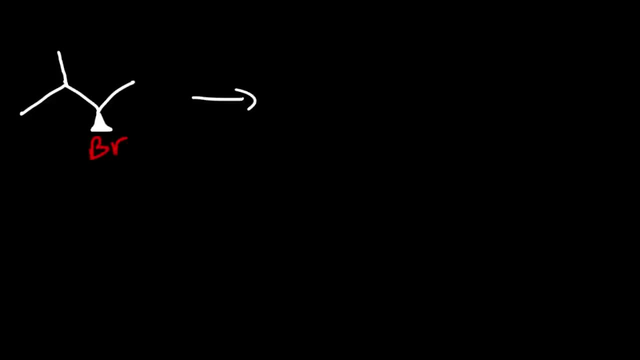 And we're going to react it with water. Now let's compare this to 2-bromo-butane And we're going to react this molecule with the acetate ion, Which is going to be dissolved in acetic acid. So go ahead and determine the substitution mechanisms. 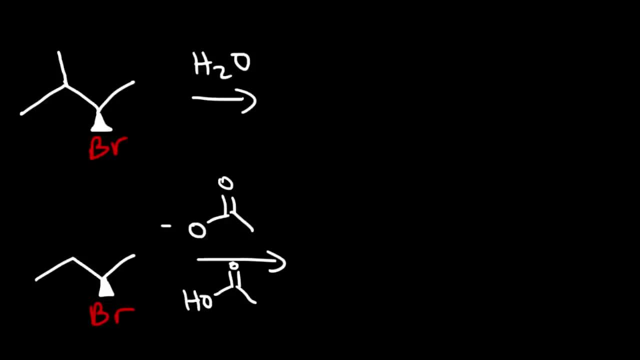 that these two reactions will proceed by Ignore the elimination mechanism. Now let's focus on the reaction on the bottom. So we have a secondary alkyl halide and a protic solvent. So if we use the chart, this would indicate that it should proceed by the SN1 mechanism. 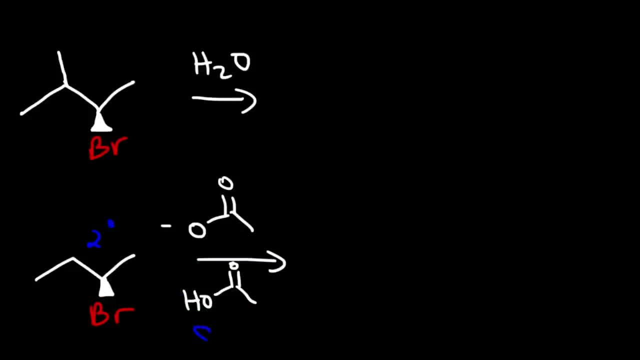 However, it turns out that this reaction actually goes by the SN2 mechanism, And for one reason. acetate is a decent nucleophile: It has a negative charge, So it's more nucleophilic than H2O. Here we have a secondary alkyl halide and a protic solvent. 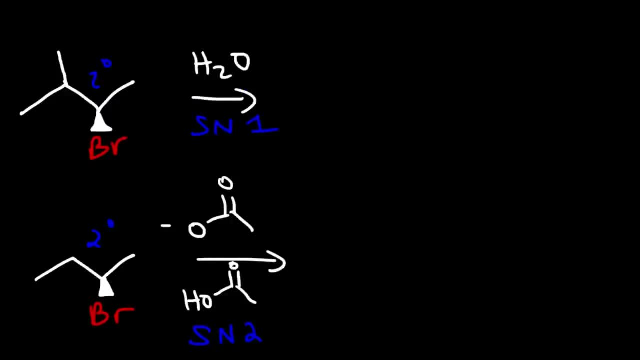 And it turns out that this mechanism favors the SN1, or this reaction favors the SN1 mechanism. Now let's talk about why. So, as we said before, we have a better nucleophile, And so that favors the SN2 reaction. The nucleophile has a negative charge. 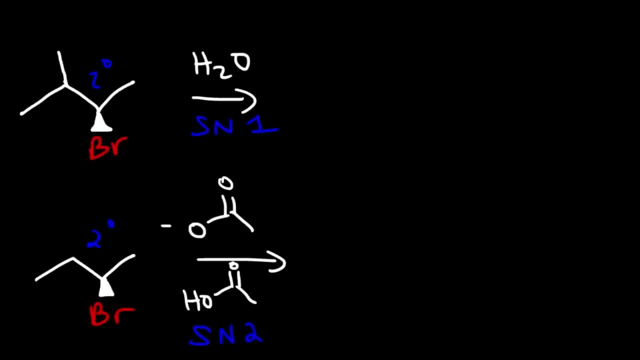 Whereas this nucleophile is neutral, Even though both solvents are protic. Now, the second reason why this one favors an SN2 reaction is because that substrate is not sterically hindered. Here we have a sterically hindered secondary alkyl halide. 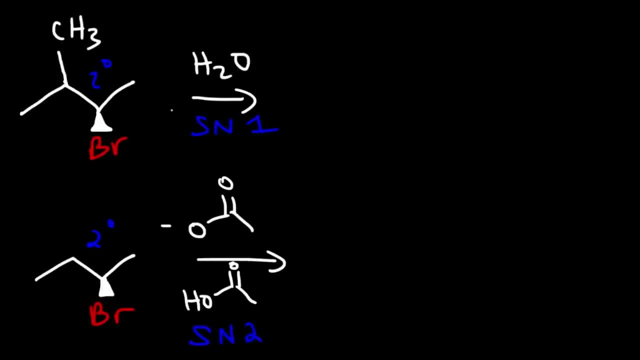 Due to this methyl group And this sterically hindered secondary alkyl halide actually favors the SN1 reaction because once we get the secondary carbocation, it can rearrange and form a more stable tertiary carbocation. So whenever you're dealing with secondary alkyl halides, 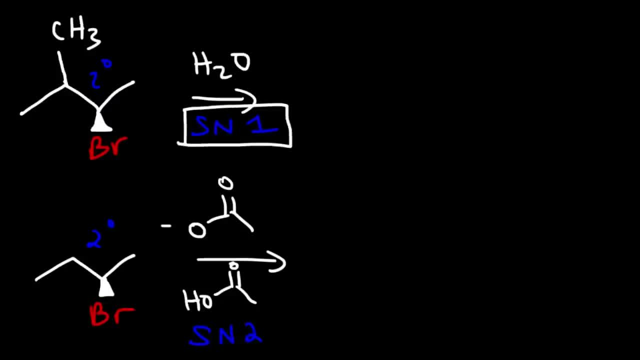 you need to be careful because sometimes it can be SN1.. Sometimes it can be SN2.. Now we know it's not going to be an E2 reaction because we don't have a strong base, So we can ignore that option. But when you're between, 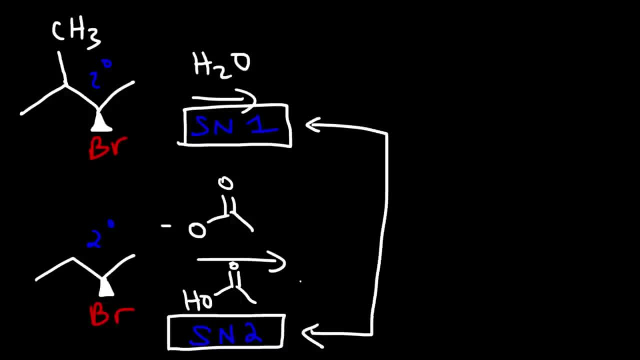 these two mechanisms. ask yourself: what type of secondary alkyl halide do I have? Is this sterically hindered? If it is, it's going to favor the SN1 mechanism. If it's not, it favors the SN2 mechanism. Is there a protic solvent or is there an aprotic solvent? 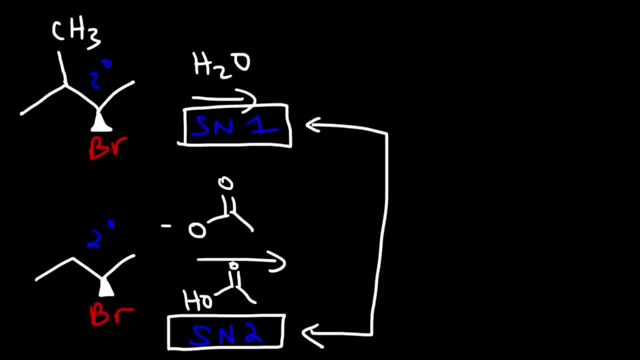 If there's an aprotic solvent, it favors the SN2 reaction. If there's a protic solvent, typically it favors the SN1 mechanism. But in this case- this exception- we have a good nucleophile in a protic solvent. so 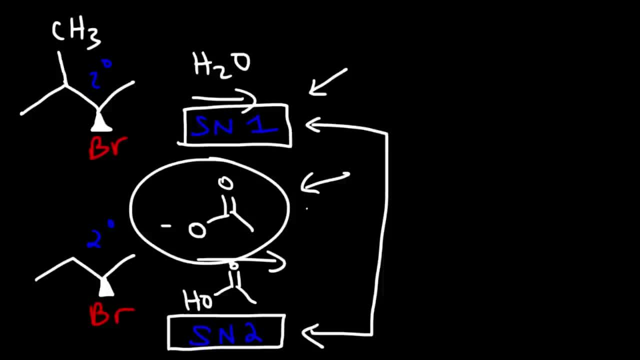 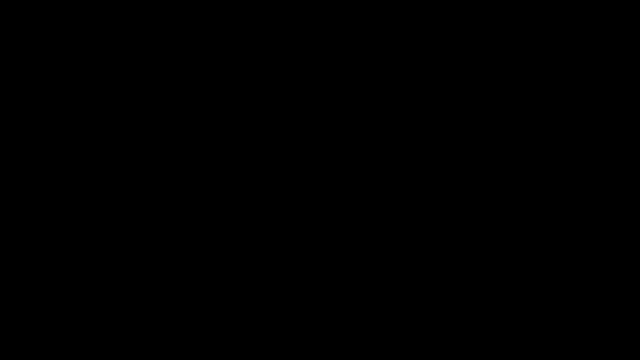 that good nucleophile favors the SN2 mechanism, And so you have to look at every detail and weigh all your options carefully. Now let's go over the mechanism of those two reactions. So let's start with this one, where we're going to react it with H2O. 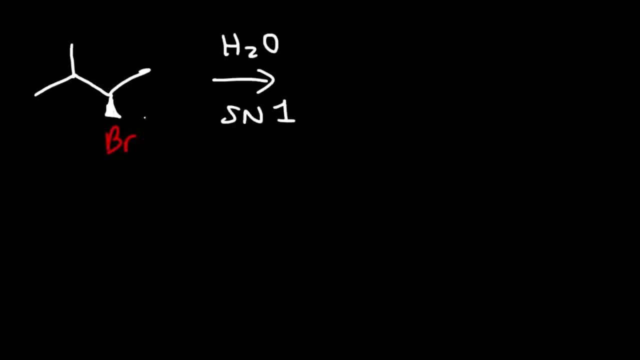 And we said that this is going to be the SN1 mechanism. So the first step, the leaving group leaves, And so we're going to get a secondary carbocation. Now, whenever you have a secondary carbocation next to a tertiary carbon, 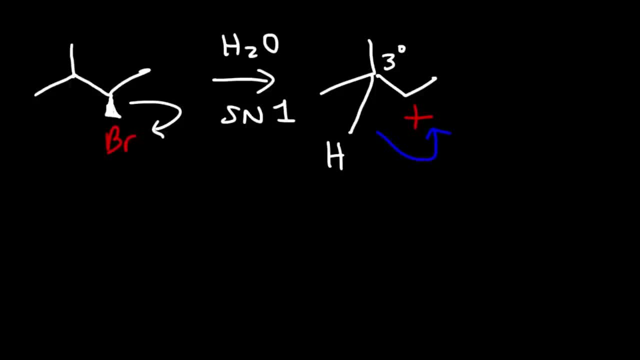 you're going to get a hydride shift, And so this is going to give us a more stable tertiary carbocation intermediate, And so water is going to attack the carbocation, giving us this intermediate, And then, in the next step, we're going to use another water molecule. 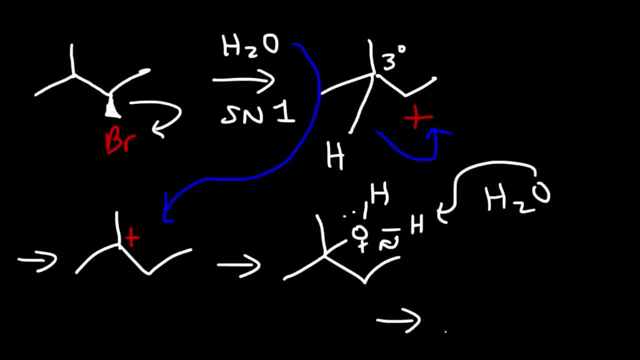 to take off a hydrogen atom, And so our final answer is a tertiary alcohol. Now, this alcohol is not chiral because it has two methyl groups, And so we don't have to worry about stereoisomers. This is going to be the major SN1 product. 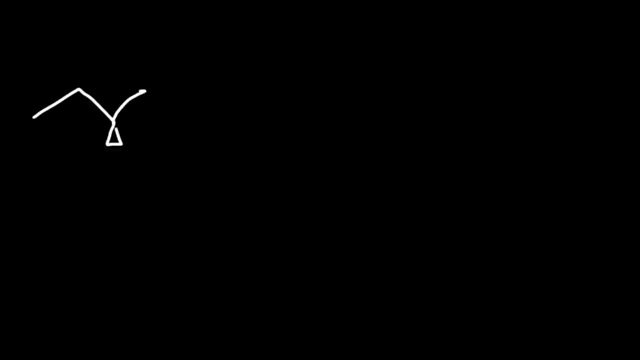 Now let's go over the other example, where we had two bromo butane reacting with the acetate ion. So we said that this reaction will proceed by the SN2 mechanism, And so the oxygen of the acetate ion is going to attack from the back. 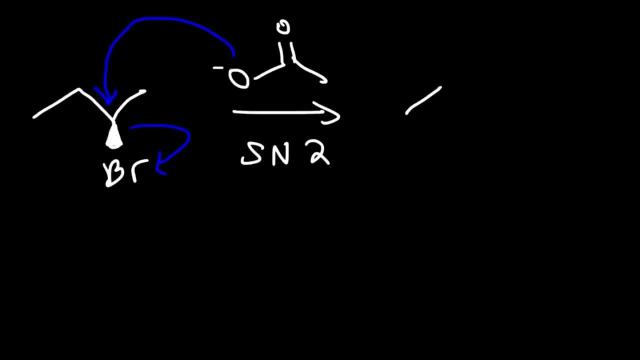 expel in the leaving group, And so we're going to get inversion of configuration. So this is going to be our product. Now here's the interesting question for you. Let's say we have this substrate and let's react it with methanol. 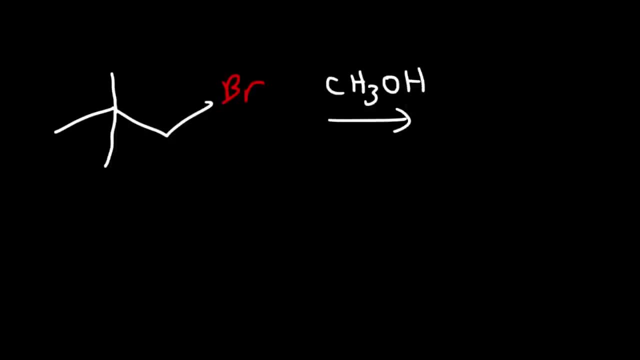 What's going to be the major product in this reaction And what type of mechanism do we have? Is it the SN2 mechanism, the E2 mechanism, SN1, E1?? What's going on here? So the carbon that has the bromine atom. 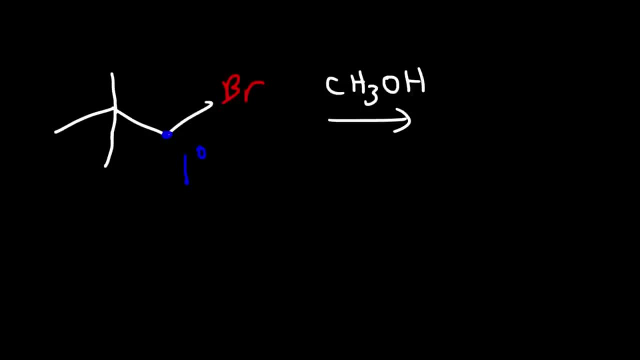 is the primary carbon. So we have a primary alkyl halide, which usually favors SN2 reactions, And we have a protic solvent, So are we going to get an SN2 reaction. Notice that this primary alkyl halide is very hindered. 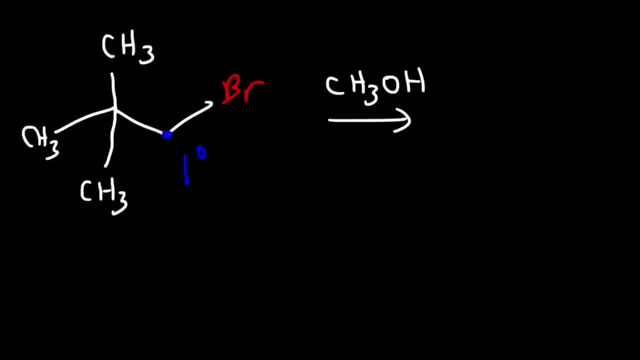 Next to the primary carbon, we have a quaternary carbon, And so, due to the fact that this primary carbon is sterically hindered due to the adjacent carbon, it's safe to say that this reaction will not proceed by the SN2 mechanism. 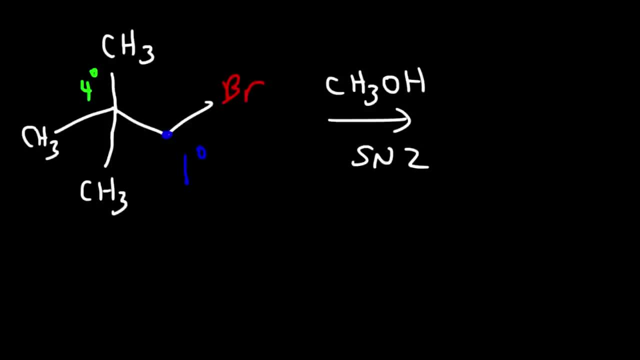 It's too sterically hindered. So what's going to happen? Can it proceed by the SN1 mechanism? It can. However, we can't just kick out the Br, Because if we do, we're going to get a primary carbocation. 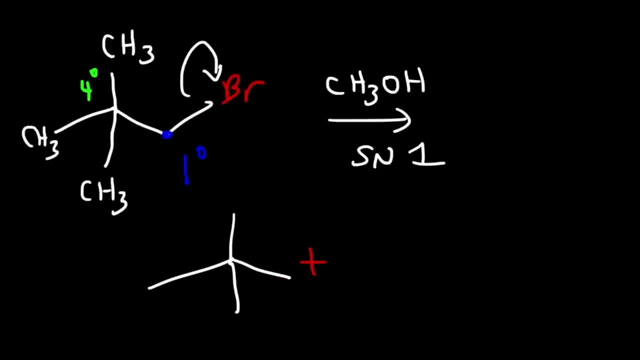 And primary carbocations are not stable, They're very difficult to form, And so that's not going to happen. Instead, we're going to get a concerted reaction. We're going to get a methyl shift before the Br leaves to produce the unstable carbocani. 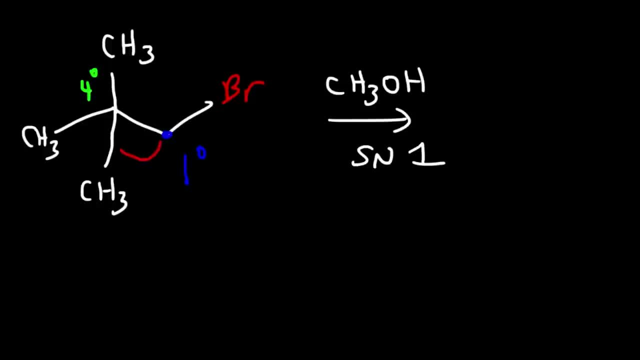 So this methyl group is going to attack this carbon, kicking out the Br atom. And so now the methyl group is here. By doing this, we form a more stable tertiary carbocation intermediate without forming a primary unstable carbocation. So now, at this point, 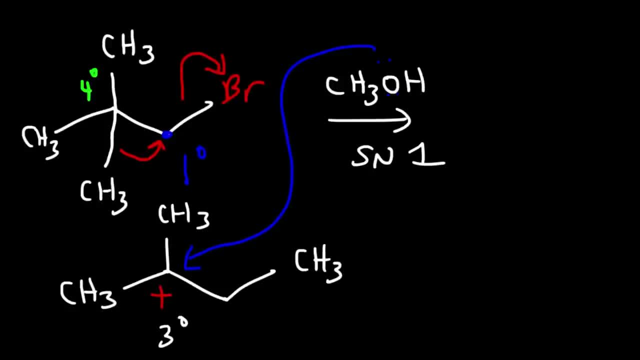 the methanol could attack the carbocation, giving us this intermediate, And then, in the next step, we can use another methanol molecule to remove the hydrogen atom, And so our final product is an ether, And we don't have to worry about. 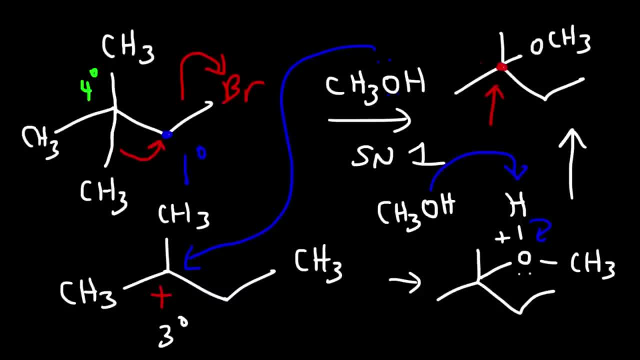 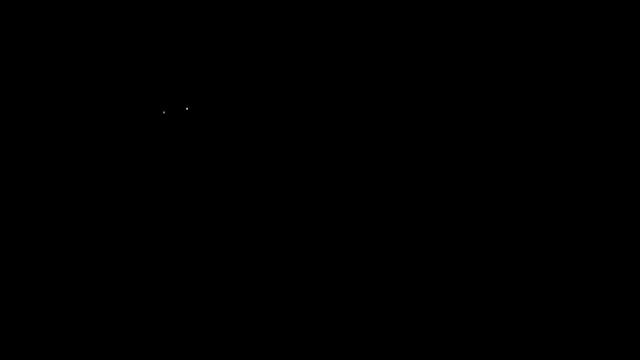 stereochemistry. This is not a chiral center, And so this is the answer. So this is one of those rare situations where a sterically hindered primary alkyl halide can give you the SN1 mechanism. Now let's consider this example. 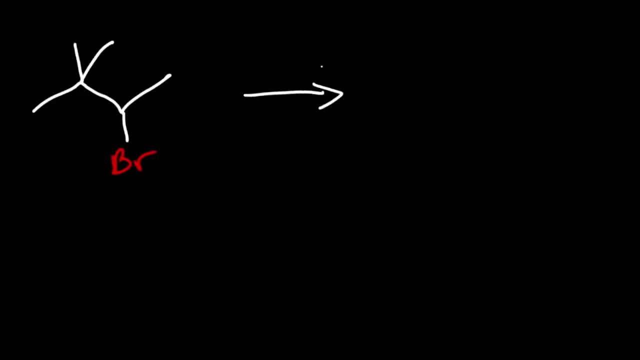 So once again we have another sterically hindered secondary alkyl halide, But this time we're going to react it with sodium ethoxide and ethanol. So go ahead and try this problem. So we have a strong base, that's ethoxide. 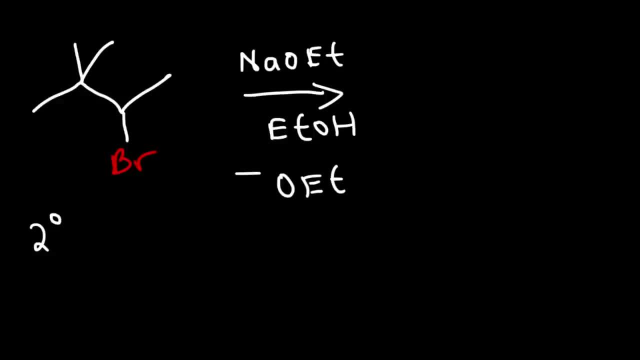 And, based on the chart, when you have a strong base like ethoxide and a secondary alkyl halide, it can predominantly give you the E2 reaction mechanism, But it can also give you the SN2 reaction. However, we do have a secondary 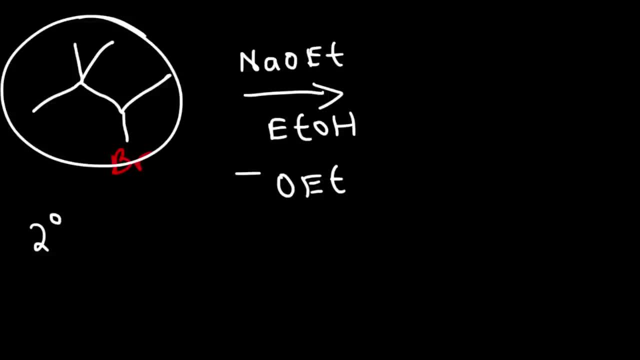 sterically hindered halide, And so we could say that the SN2 reaction is negligible. If it does occur, it's going to be in a very, very low yield. So we're going to ignore the SN2 reaction And we're going to focus. 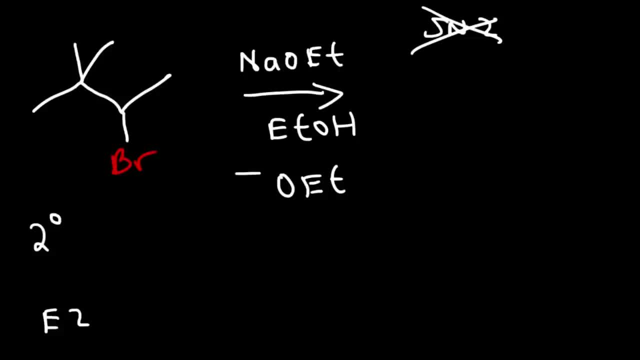 on the E2 reaction, Because that's going to be the dominant mechanism if you have a sterically hindered substrate, So notice that we can't get the Zeta product. in this case There is no hydrogen on its carbon because it's quaternary. 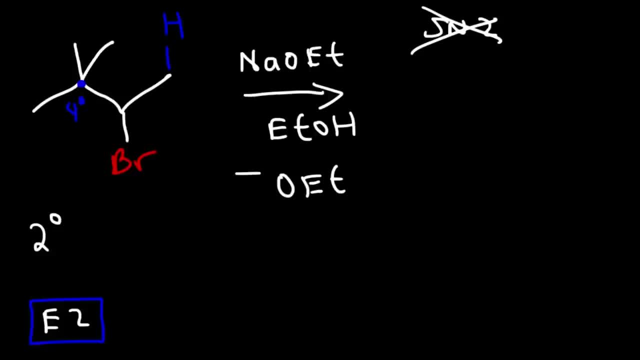 So we have to remove the hydrogen on the primary carbon because we have no choice, And so ethoxide will go for this hydrogen and we can only get one product. For the E2 reaction, there are no rearrangements, And so this is one of those rare cases where 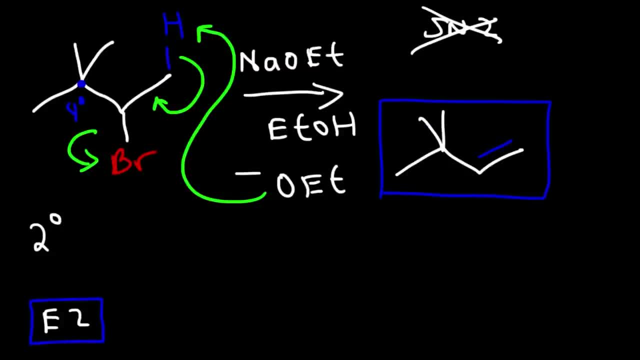 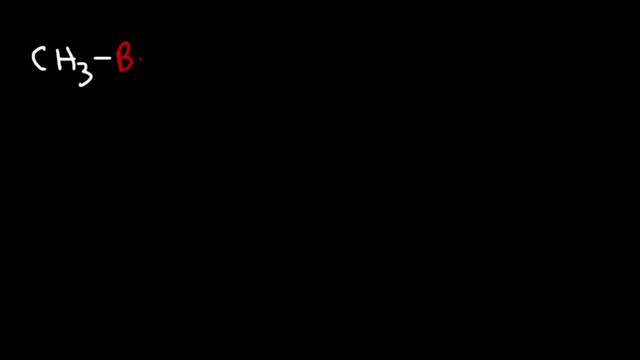 we get the less stable alkene. since we only have one choice, We have no other choices, And so that's it for this example. What's going to happen if we mix methyl bromide with terpitoxide? Go ahead and predict the product of this reaction. 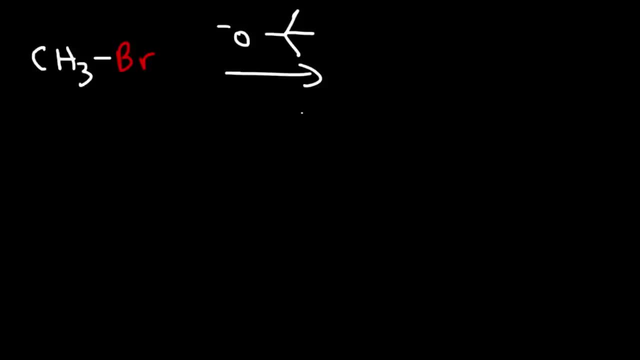 Now, whenever you have a methyl substrate, the only mechanism that can work is the SN2 mechanism. There are no other choices. Now, even though we have a bulky base such as terpitoxide, which typically favors elimination reactions over substitution reactions, we can't form a double bond with 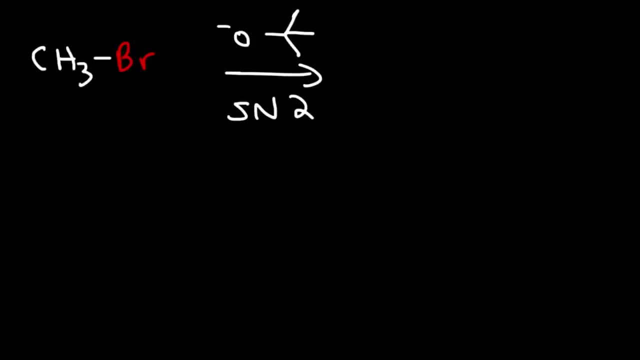 one carbon atom. You need at least two carbon atoms to form a double bond, And so there's no way we can get the E2 reaction. So the SN2 reaction will occur with a 100% yield. So what I'm going to do is draw the terpitoxide. 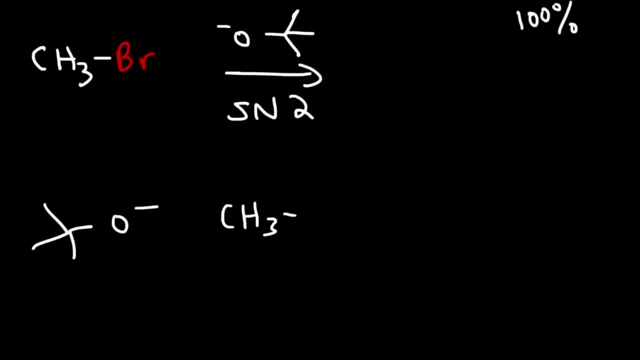 first and then the substrate after that. So terpitoxide will attack the methyl group from the back and expel in the bromide ion, And so our product will be an ether, And so this is the only product that we can get in this reaction. 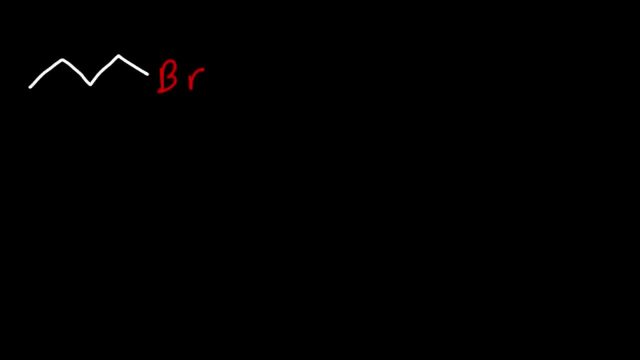 Now let's move on to this example. So here we have butyl bromide and we're going to react it with methoxide and methanol. So, based on the chart, if we have a primary alkyl halide, that's not sterically hindered. 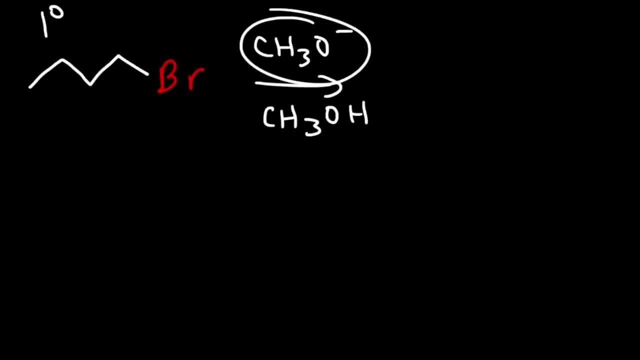 and we have a strong base. what is going to be the dominant mechanism in this reaction? So, since we don't have a sterically hindered base, the mechanism will predominantly be SN2.. And so, in this case, the methoxide ion will attack the carbon. 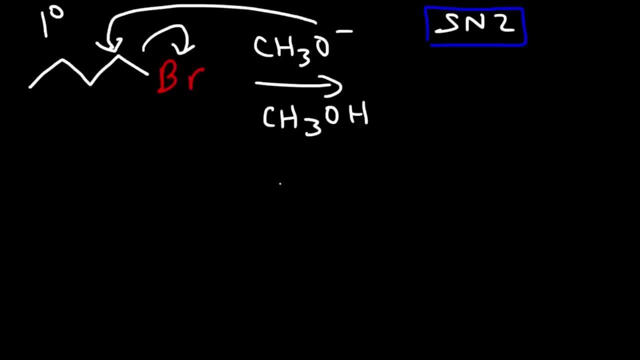 that bears the bromine from the back, expelling the leaving group, And so we're going to get an ether. Now we don't have to worry about stereochemistry, because this carbon is not chiral. It has two hydrogen atoms, And so that's. 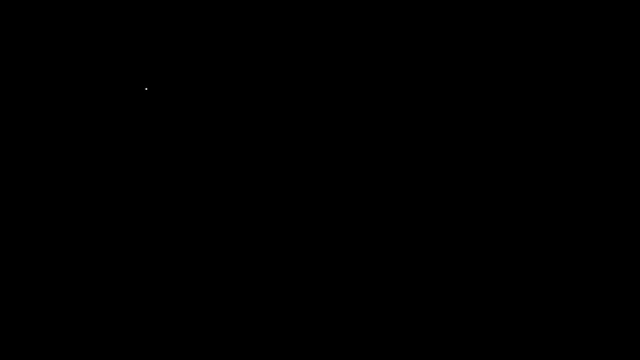 it for that example. Now, what if we have a primary alkyl halide, but with a sterically hindered base like terbutoxide? What's going to happen in this case? Well, based on the chart, this is going to favor the E2 reaction. 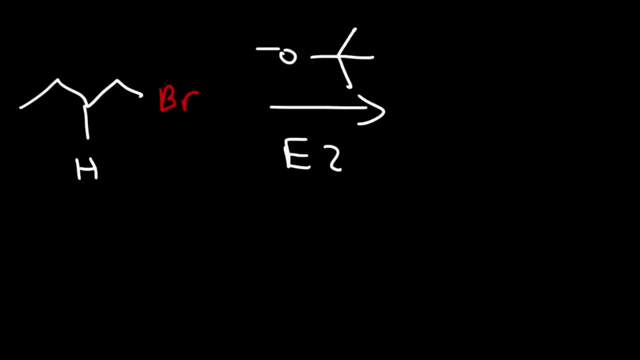 So the base, this bulky base, it doesn't like to behave as a nucleophile because it's so bulky- Unless it has to in the case of methyl bromide- But it prefers to behave as a base abstracting a proton. And so this is going to give us. 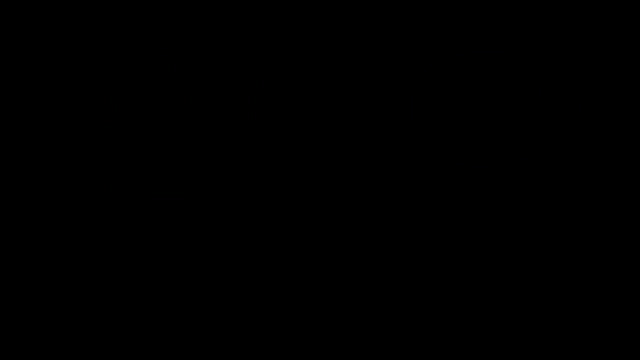 one butene. Now I want to compare the last two reactions with a new reaction, And so you can see something. So here we have a primary alkyl halide with an unhindered strong base, And so this gave us the SN2 reaction. 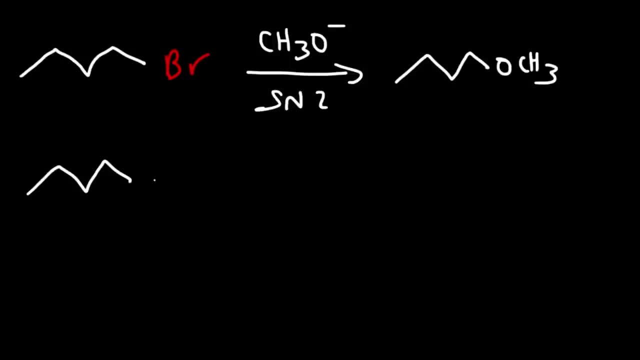 In the last example, we had a primary alkyl halide that was not sterically hindered, but we had a sterically hindered base, And so this gave us the E2 reaction. Now, what if we have, let's say, a sterically? 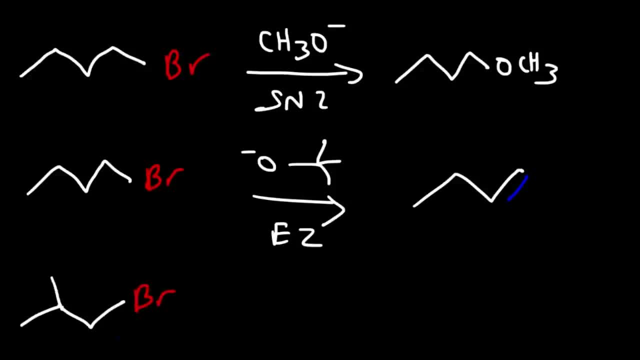 hindered primary alkyl halide And let's use methoxide again, Will we get an SN2 reaction or an E2 reaction? So in the first example, if we don't have a sterically hindered base or a sterically hindered primary alkyl halide, 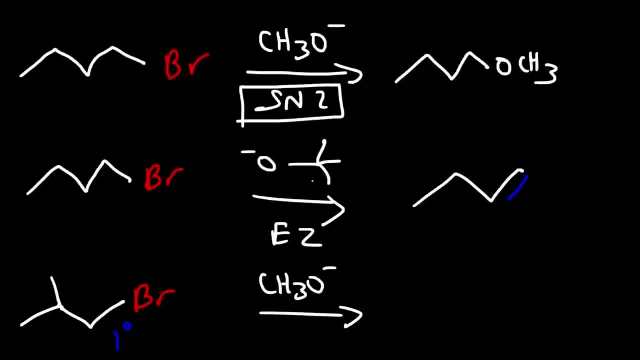 we get the SN2 reaction. If we have a sterically hindered base, we're going to get the E2 reaction. If we have a primary sterically hindered substrate, we're going to get the E2 reaction as well, Because any time 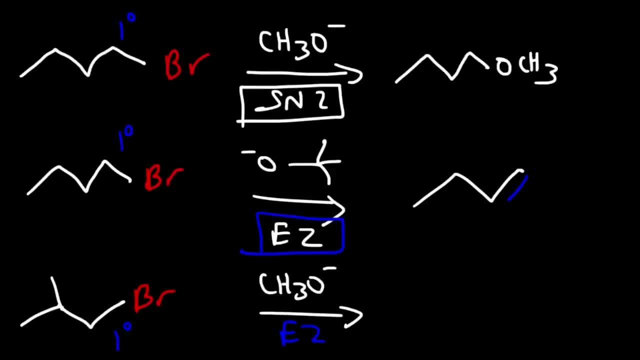 you have a sterically hindered substrate, it's going to weaken the yield of the SN2 reaction And so therefore, we're going to get this alkene. So make sure you understand that. So the only time you get the SN2 reaction. 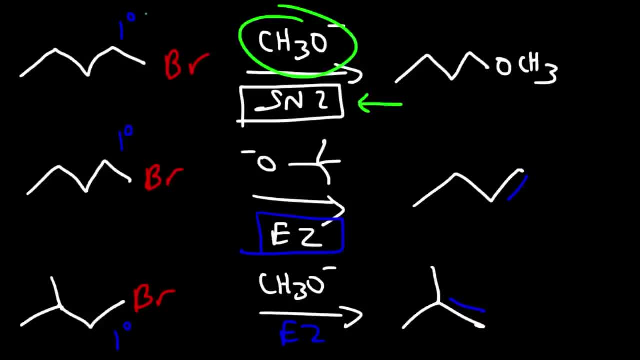 with a strong base is if you have a primary alkyl halide that is not sterically hindered. If you have a sterically hindered base or a sterically hindered primary alkyl halide, it's going to favor the E2 reaction. 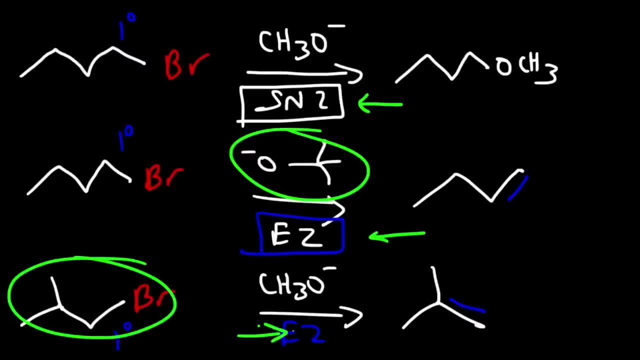 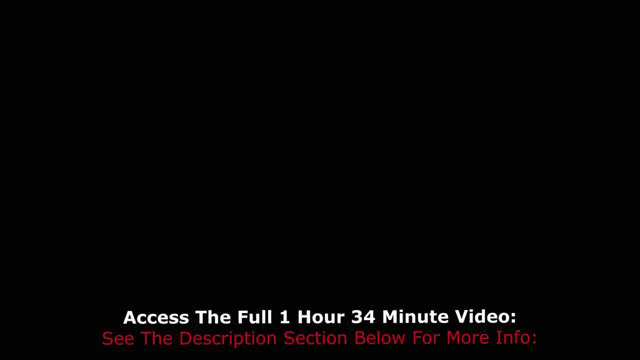 over the SN2 reaction. You can still get the SN2 reaction, but the E2 reaction will give you the major product. Thank you,